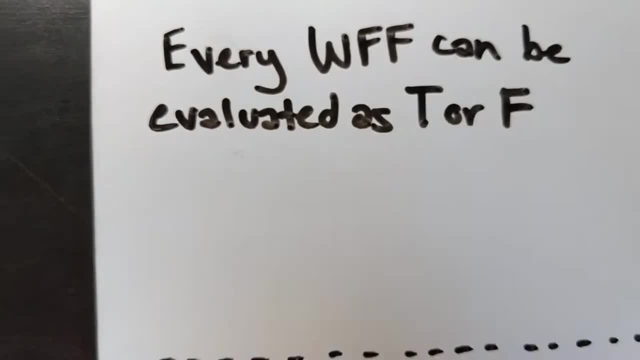 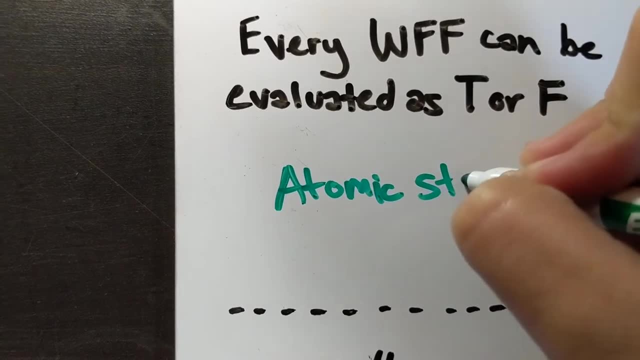 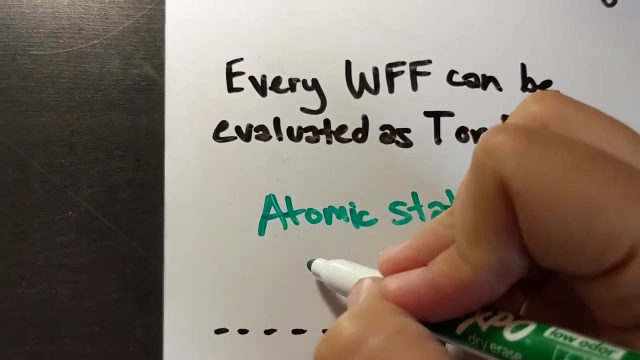 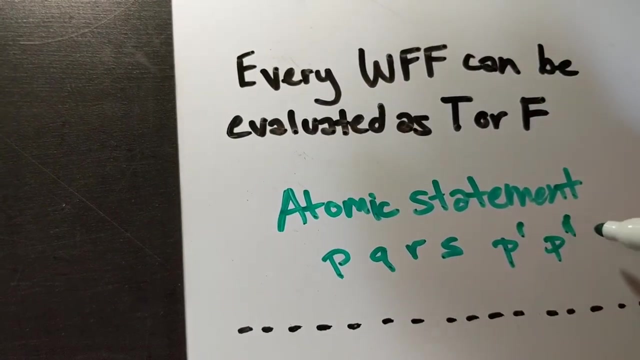 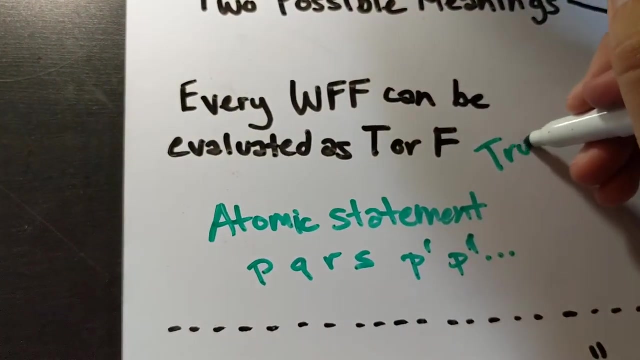 to be evaluated as true or false, and our most basic type of well-formed formula is an atomic statement, and that means that every atomic statement- remember, these are P, Q, R, S, P, prime, P, double prime, so on and so forth- has to be assigned a truth value. that's what we call these. we call these truth values. 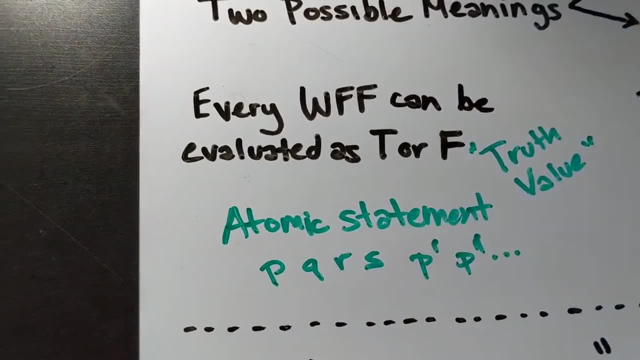 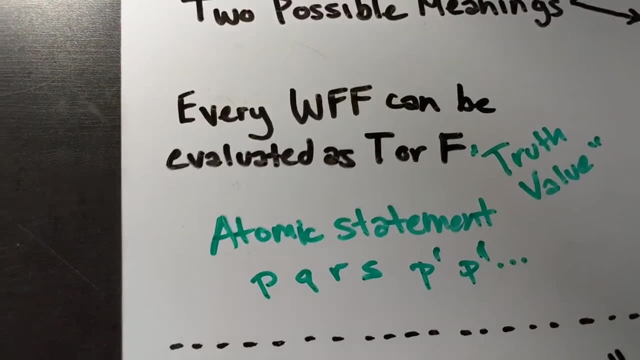 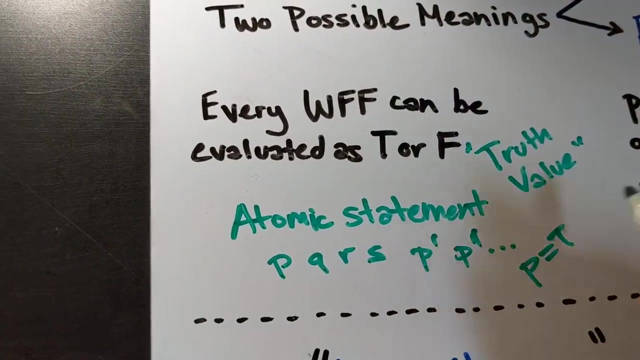 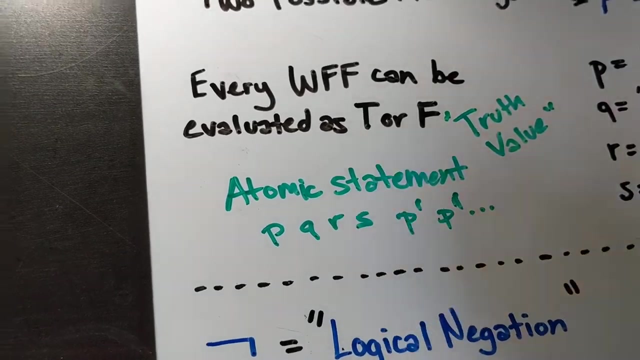 right. so every atomic statement has a truth value, and so we can think of atomic statements either as just simply P equals T, right, P equals T. that doesn't give us that much power to explain anything in the real world, but we can think of an atomic statement is essentially being a variable standing in. 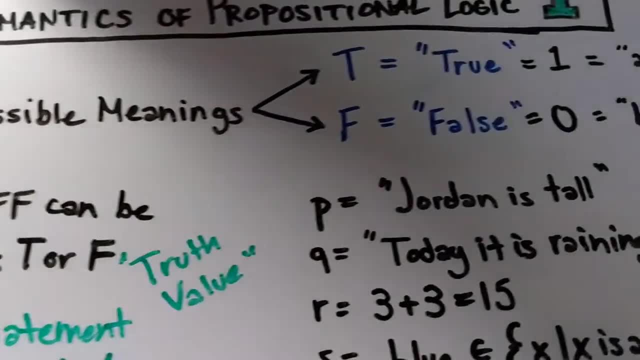 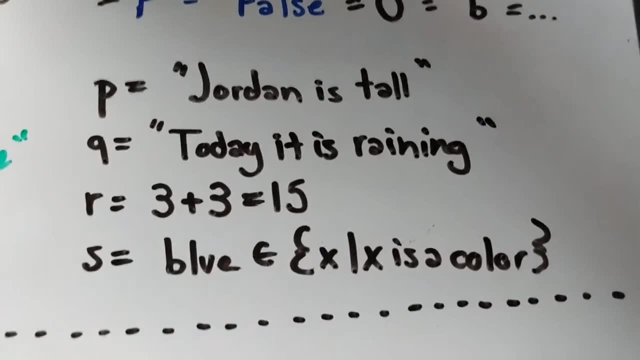 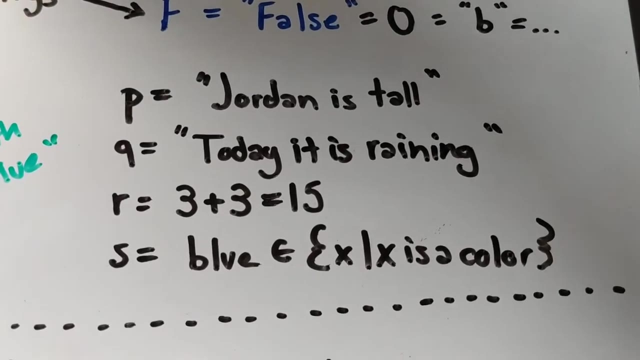 for some statement in another formal language. So, for example, P might be Jordan is tall, Q might be today it is raining. those are both in natural language, but you could have the, you could have the. the variable be standing in for something in a formal language like math. so R might be 3 plus. 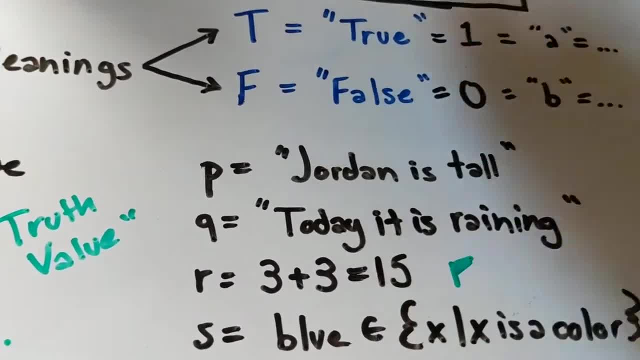 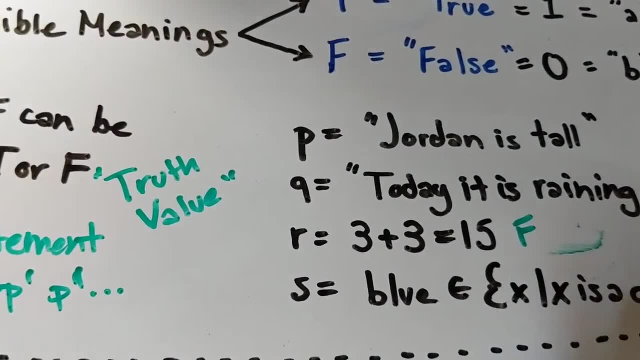 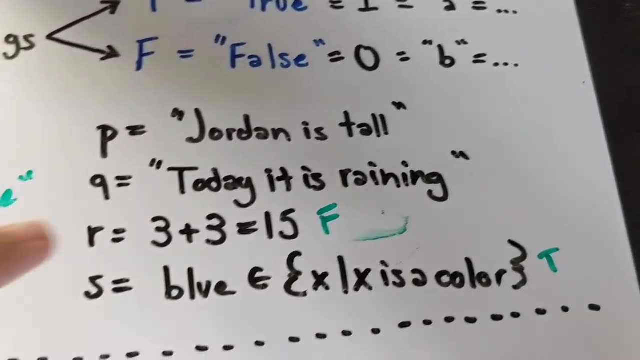 3 equals 15, which we would evaluate as false, right. or it could be in set theoretic notation, right. so blue is a member of the set of things X, such that X is a color which is true, right. So so think of atomic statements as essentially being variable, standing in. 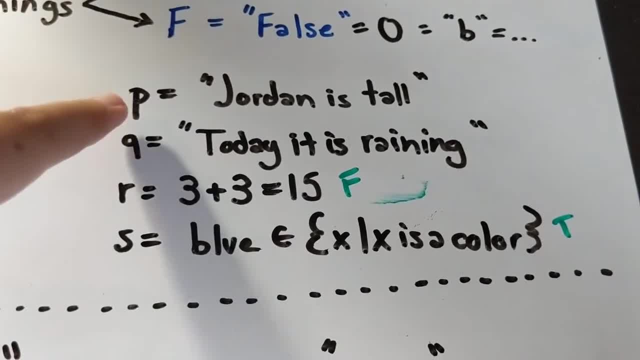 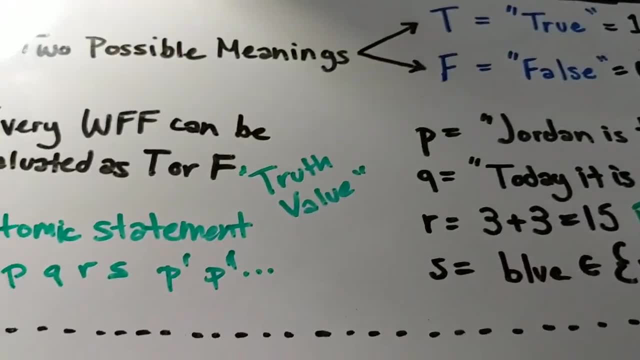 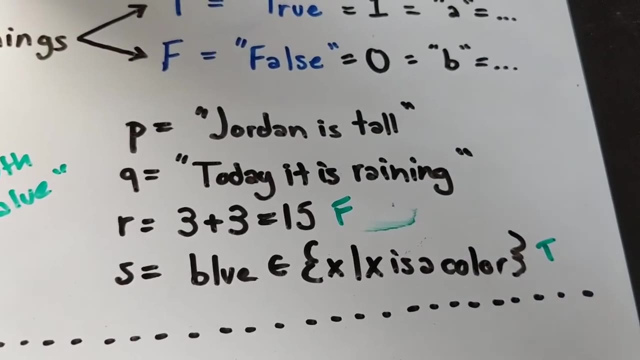 for some sort of statement, and this is why you might want to have a bunch of different atomic statements instead of just using T and F directly. right, so why you would? you need something to stand in for T and F, because really they're standing in for a statement in some other formal language which you can. 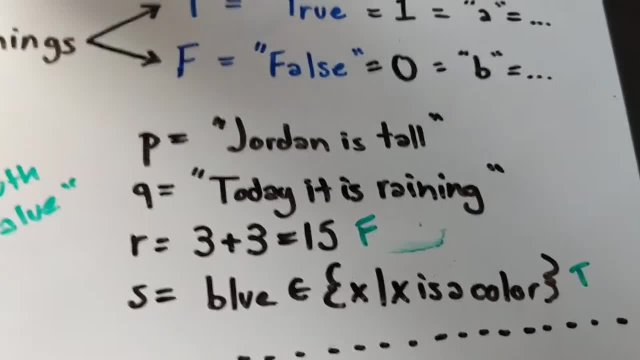 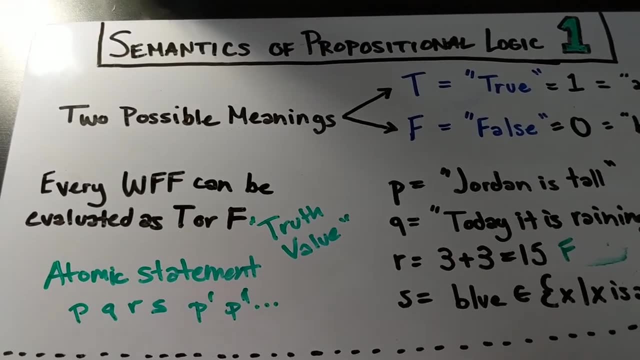 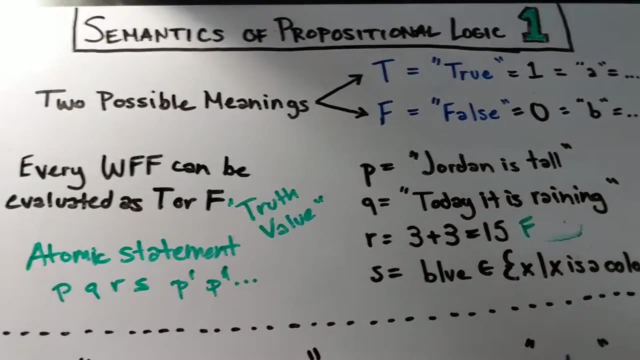 evaluate as being true or false. right. so this is a, this is the. this is the basics of the semantics of atomic statements. but well-formed formulae aren't restricted to atomic statements. right, you can combine them with other symbols and other well-formed formulae to make other meanings, to make more. 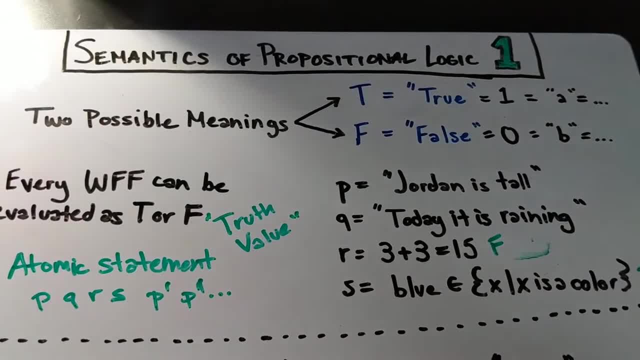 complicated statements, and that's what we're going to do in the rest of this video and the next couple of videos- is talk about combining the meanings of well-formed formulae to make more complex meanings, which we're going to talk about in the next couple of videos. 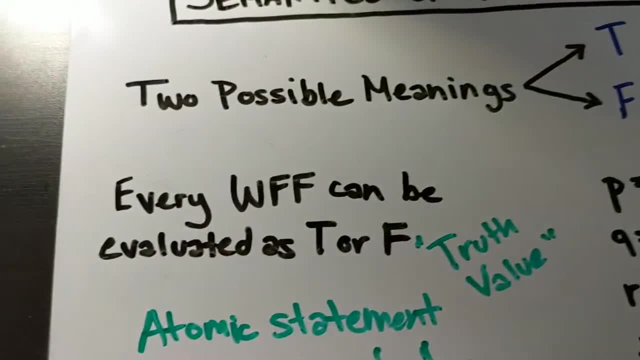 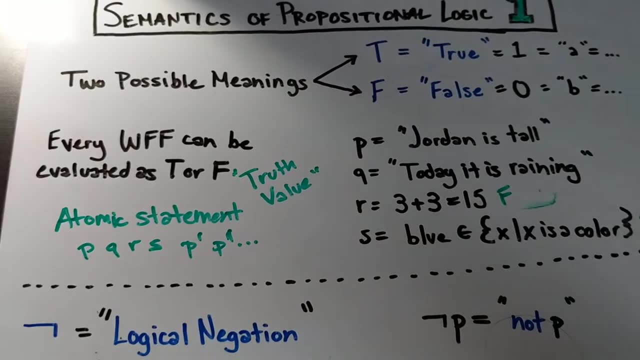 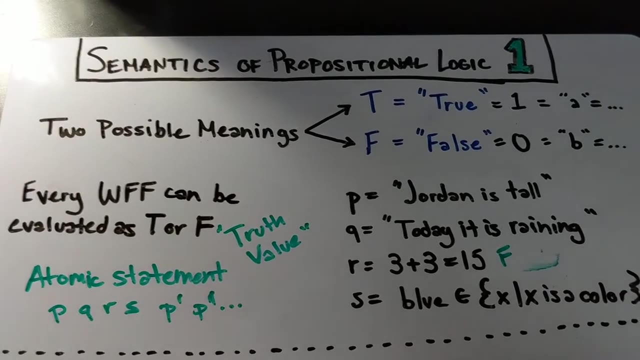 We'll always break down into true or false because, remember, every well-formed formula can be evaluated as either true or false. so it's sort of about breaking them down step by step into these meanings, just like you might do with it with solving algebra equations, right? so you might break it down until you get an. 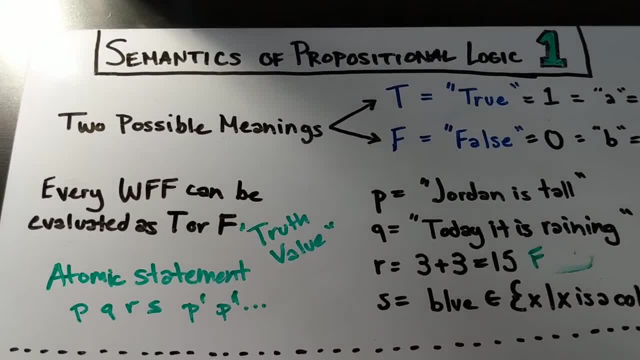 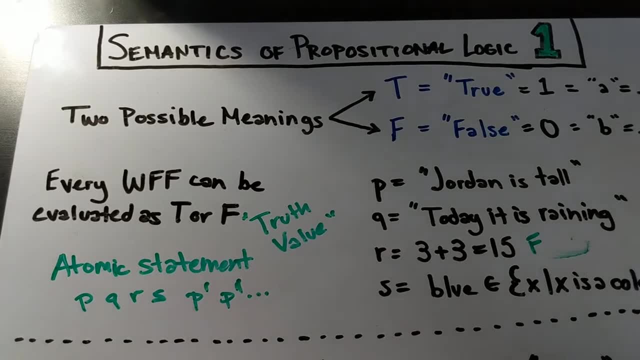 answer for X equals 7, for example. right, you can break down the meanings of complicated statements into something that is more complex than a common statement, much simpler. So our first symbol that we're going to talk about is this crook one, Remember. 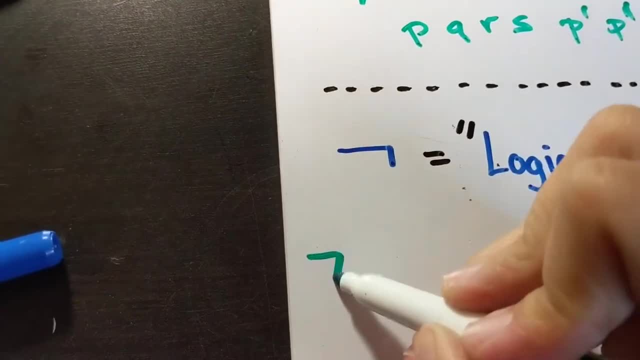 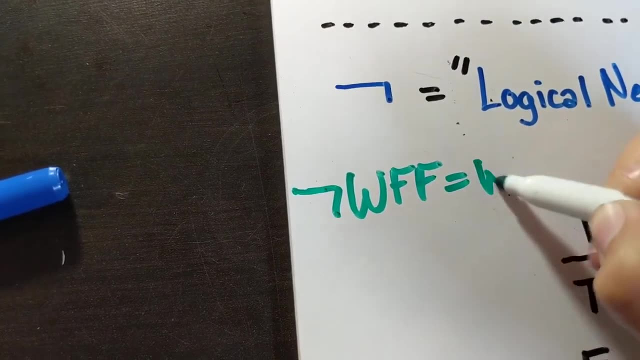 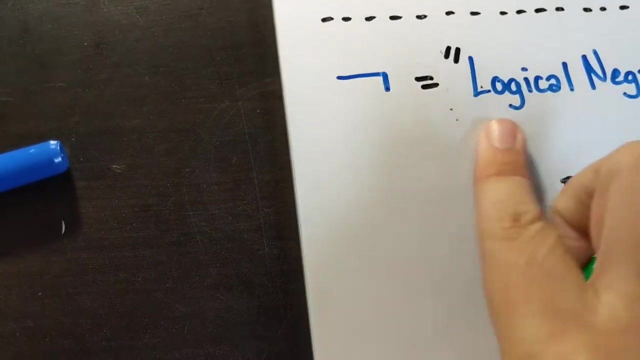 you can make a well-formed formula by taking the crook, putting it in front of a well-formed formula, and that gives you a well-formed formula. Remember from our syntax right. So this crook symbol we call logical negation And you can say negation if everybody knows you're talking about. 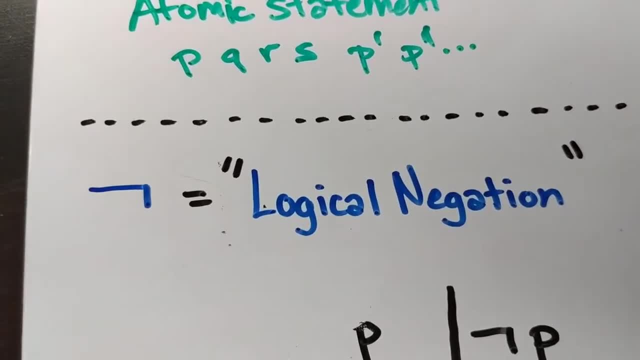 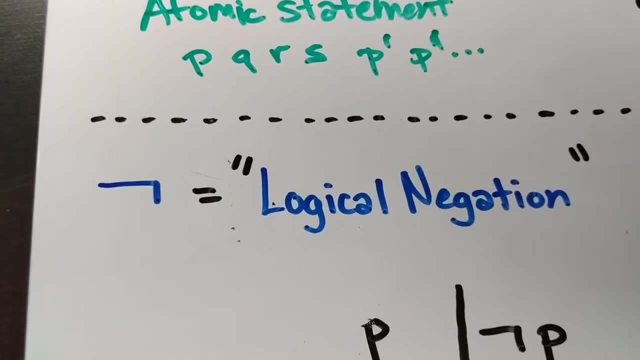 logic. We just call it logical negation because there's negation in a lot of natural languages have negation and stuff like that And it doesn't always work exactly the same way that logical negation works. So, for example, if you speak a dialect of English that has multiple negation, 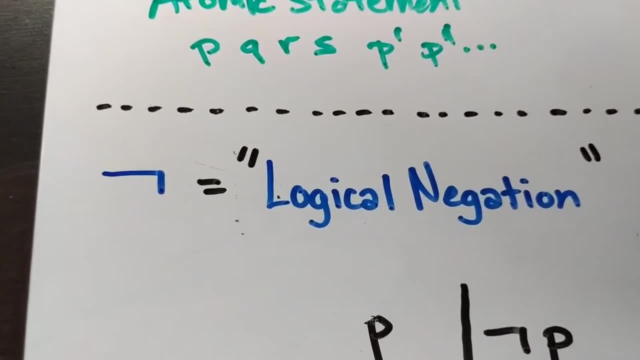 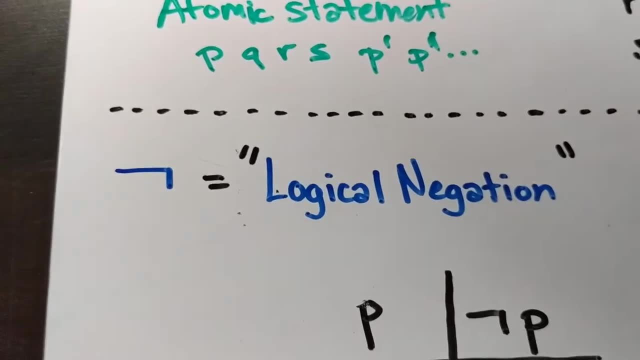 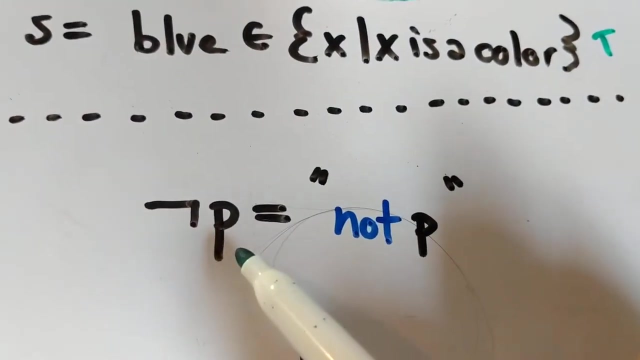 where you say: I don't never want to do that again, for example. logical negation does not work that way. Logical negation always negates every time you apply it, which we'll see in a minute. When you see a statement like this, with the crook, followed by a well-formed formula, you say: 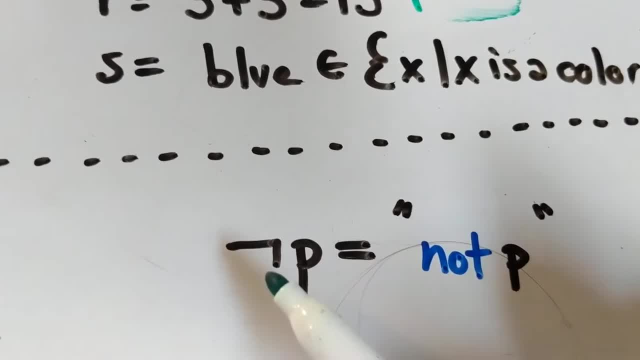 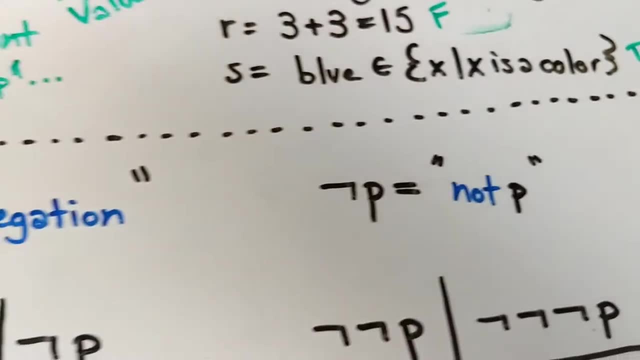 not. and then the well-formed formula. So in this case, crook P is read as not P, So that's how you read it out loud, if you're curious about that. So this is our first instance of what we call a truth table. 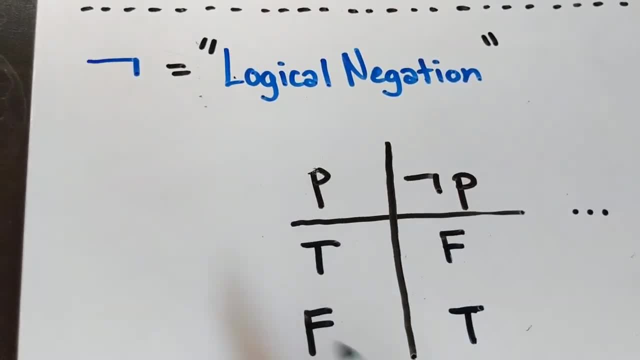 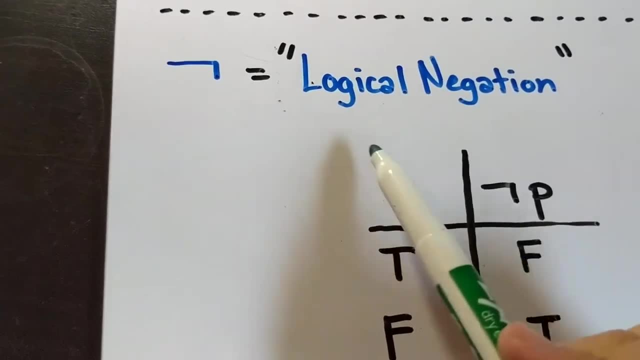 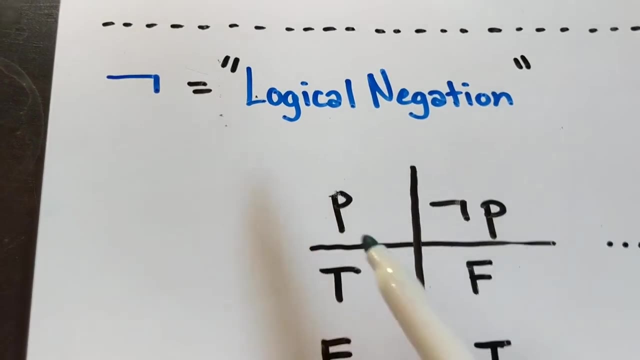 And this is a table that we can use to write out our thinking about how you determine whether something is true or false. So on the most left-hand column here we have P, which is our atomic statement in, not P. That's the atomic statement that we start with, And there's two. 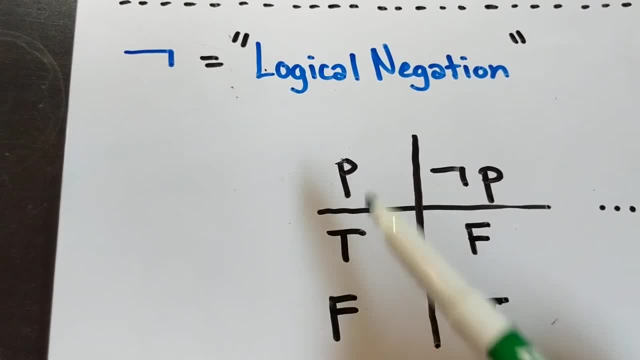 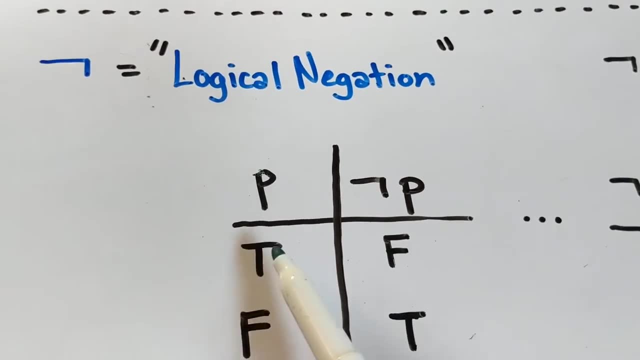 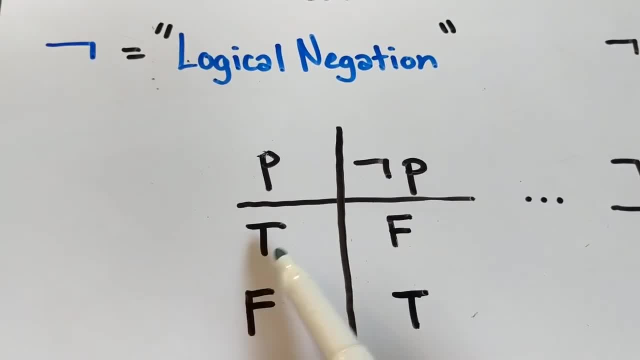 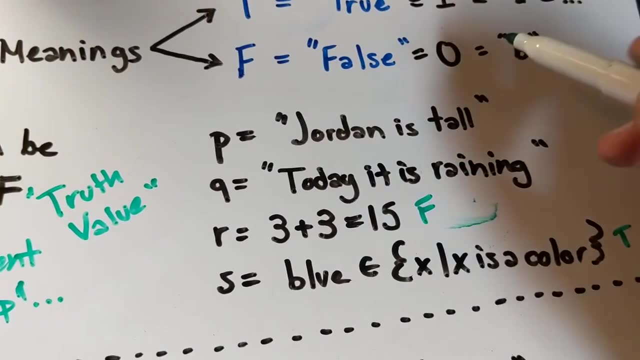 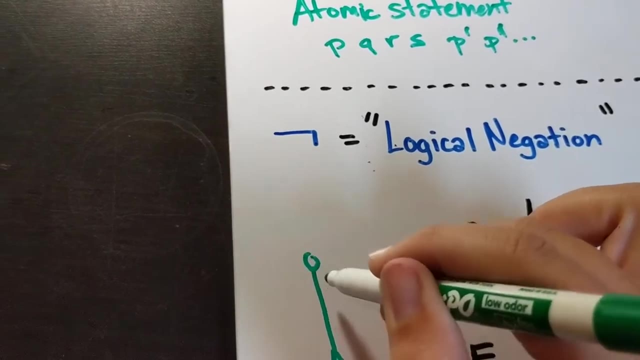 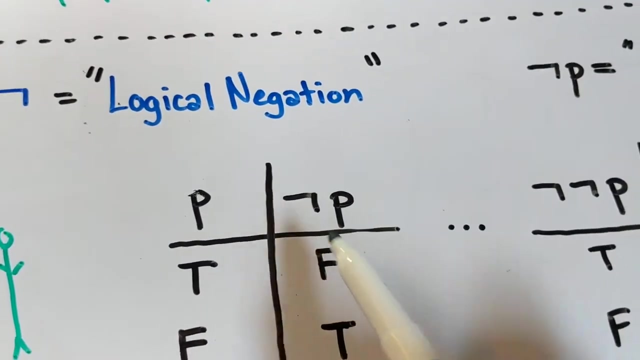 value and what happens if P has this value and we negate it. So imagine you're saying Jordan is not tall in a world where Jordan is tall. If Jordan is very tall, here's Jordan being very tall. Jordan is very tall and we say: Jordan is not tall. that statement is now false. 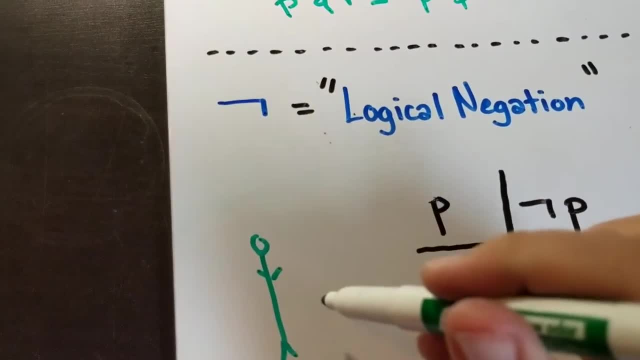 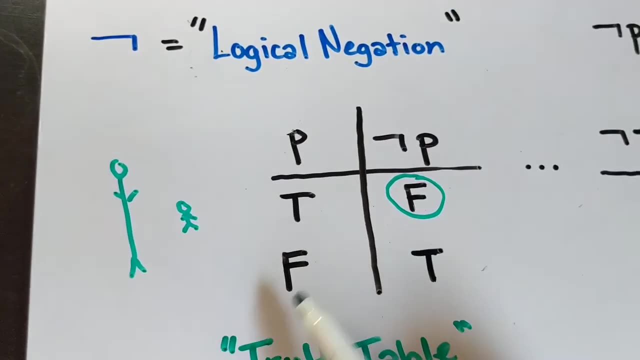 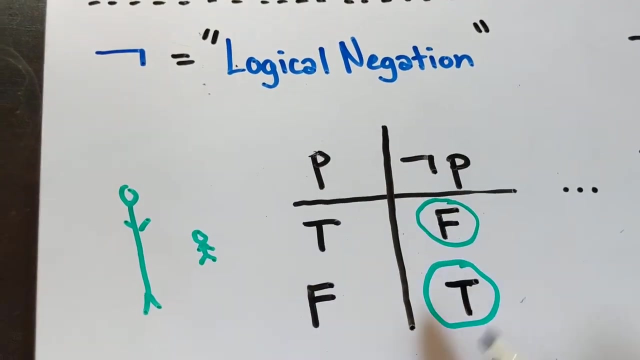 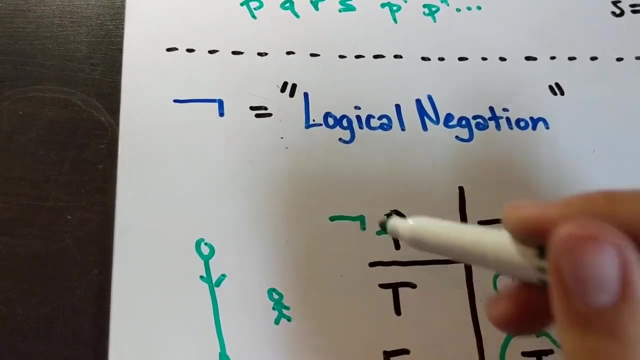 Right. In a world where Jordan is very short, here's very short Jordan and we say Jordan is tall, then that statement is false. But if we say Jordan is not tall, the statement is true, Right? So this is how logical negation works, Whatever value this well-formed formula has once you put the crook out. 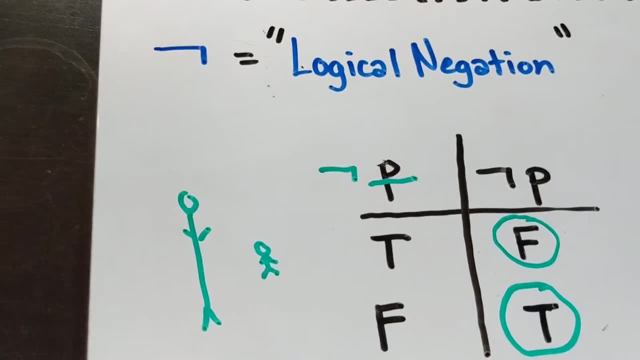 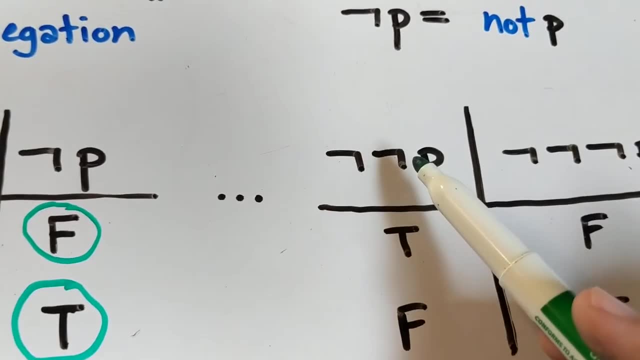 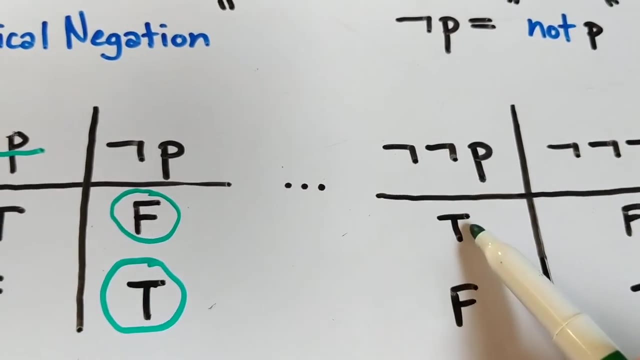 in front of it, that value just flips. Right, That value flips. So what does that mean? when we apply multiple negation of logical negation, Right Not, not P Right, So if P has the value true, not P has the value false, and then we flip that and it has the value true. 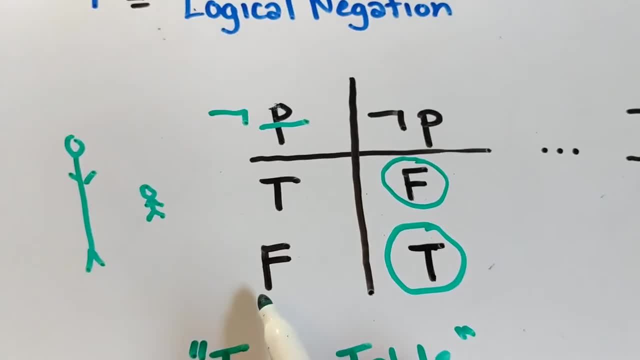 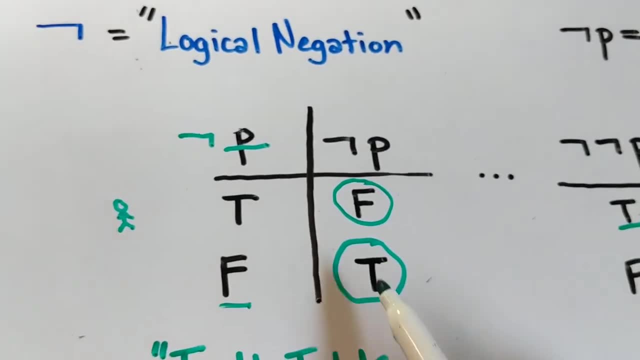 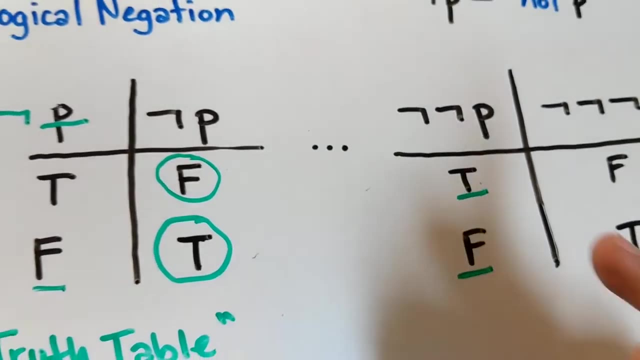 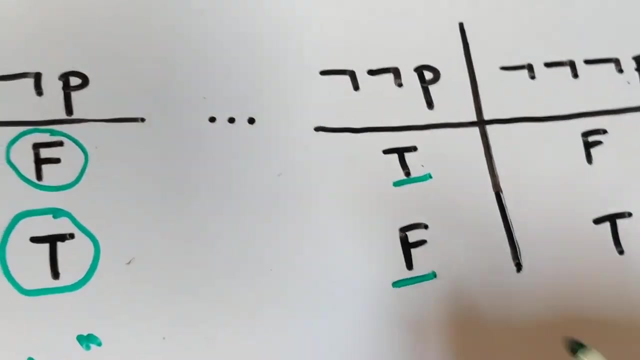 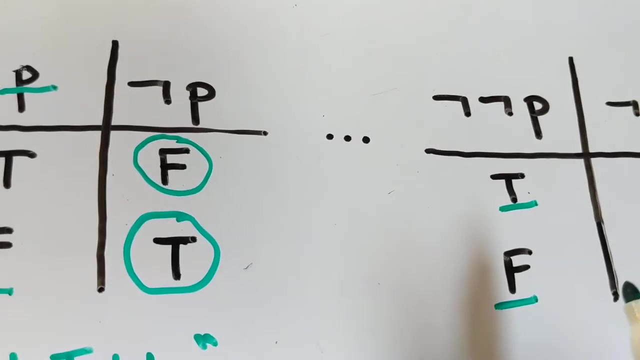 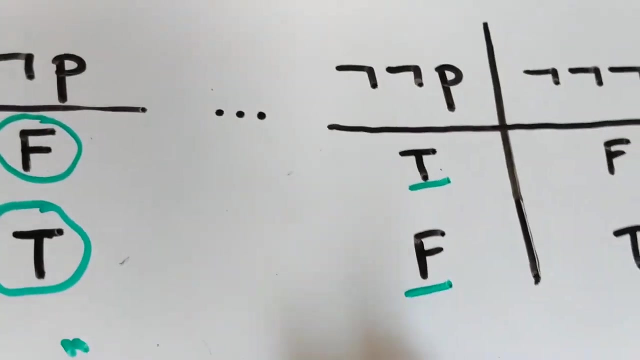 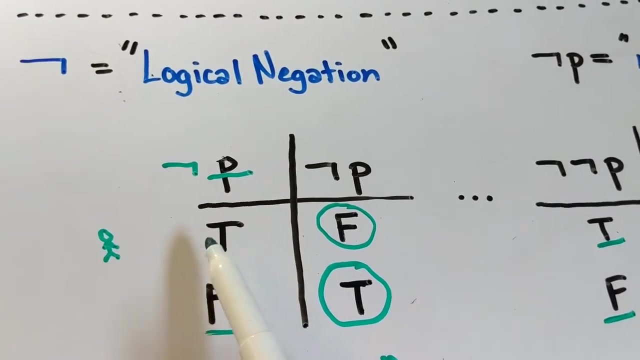 Right If P has the value false. so we say Jordan is tall. in a world where Jordan is short, right, Jordan is not tall is true. and Jordan is not not tall is false, Right. So in natural language, if Jordan is short and I say, well, Jordan's not not tall, then I'm sort of implying: Jordan is medium height or, you know, not very small, at least. Right, He's, he's, he's not. you know he might not be tall, tall but he's, you know not. not tall, Right. But this is not how logical negation works. Right. In logical negation, all that negation means is flip that, Flip it around, Right. 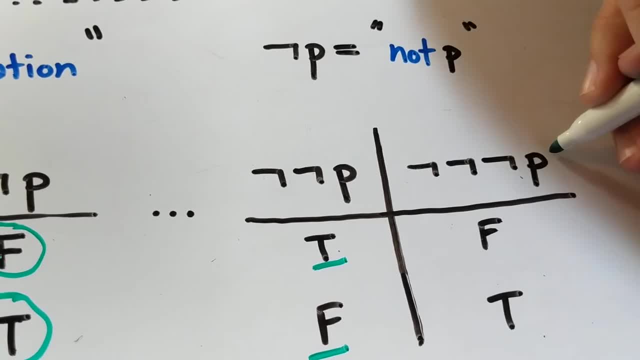 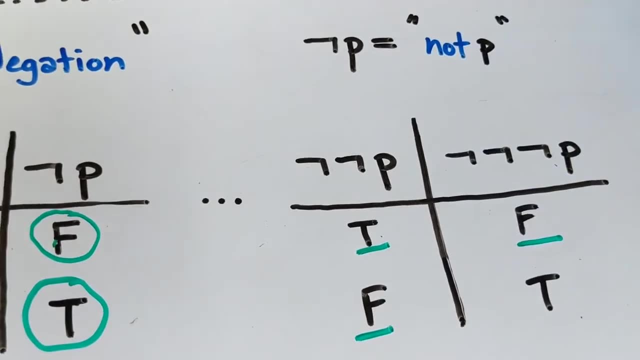 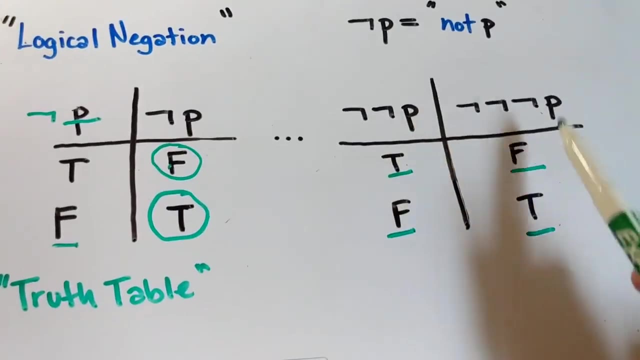 So not, not, not P Right. If P is true, then not P is false and not, not P is true and not, not, not P is false, Right, And so on and so forth. You can just keep adding negation out in front of P and you can keep computing this by flipping it every time.